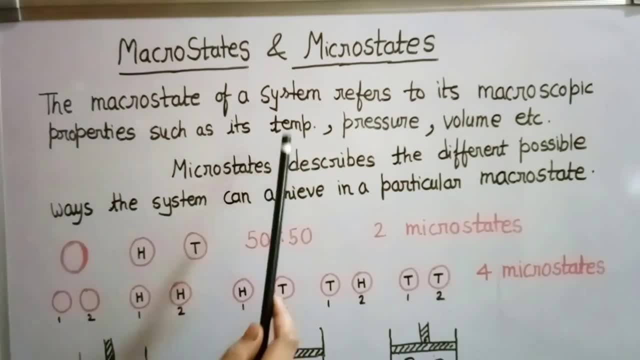 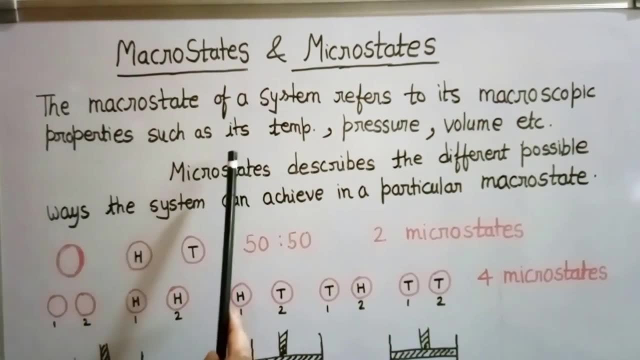 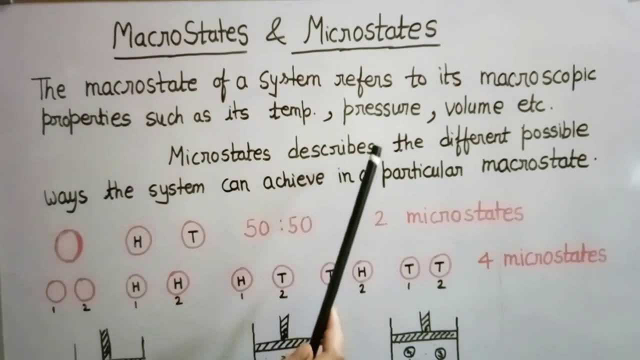 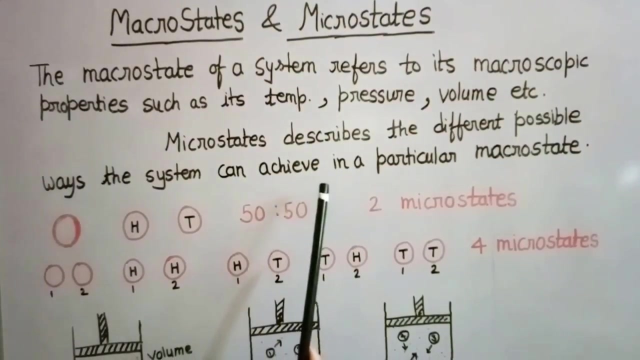 properties such as its temperature, its pressure, its volume or its number of particles. etg. these properties defines the macro state of a system, while the microstate describes the different possible ways the system can achieve in a particular macro state. now, this definitions looks so difficult. in order to understand these, 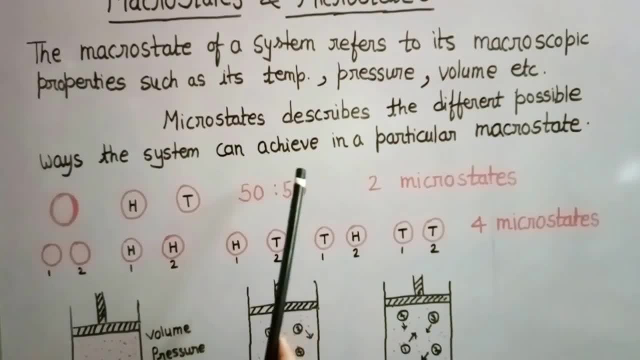 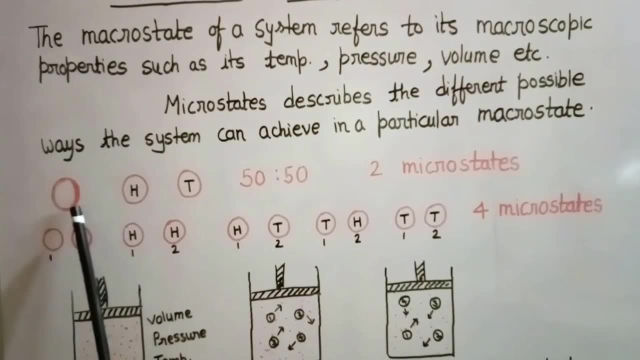 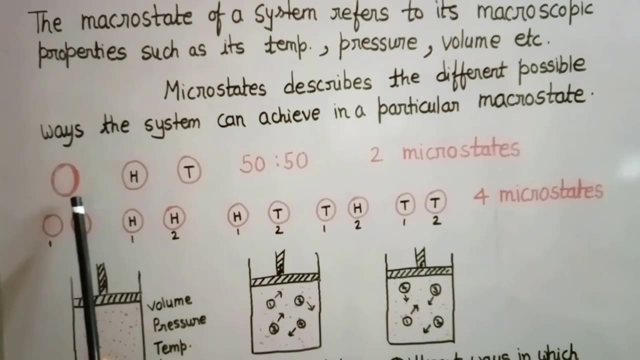 we will. firstly comes to our daily life uses. we see in our practical life some important things as we think, if we see the coin, we have a one rupee coin. when we toss this coin, what is the possibility the head will come, or what is the possibility the tail will come? 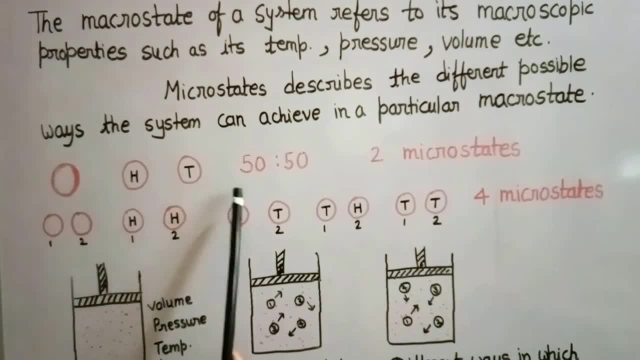 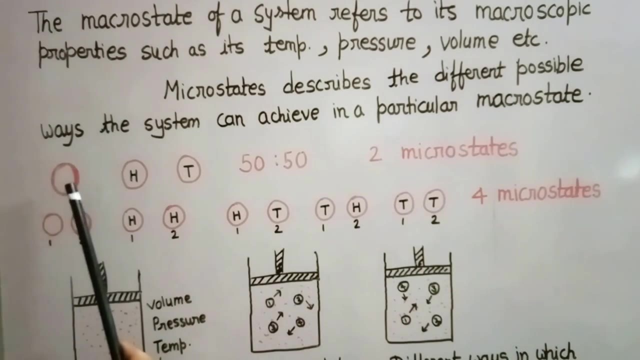 there are two equal property. it means 50: 50 property probability that the head will come or the tail will come. both have the equal probability. so this will have two microstates. the coin is one. this is the macro state and it can take the head side or it can take. 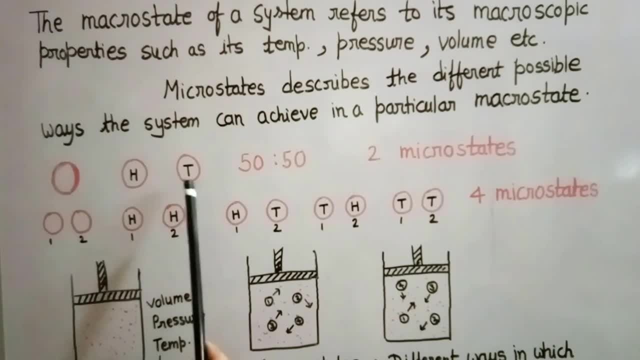 the tail side. these are two different ways that the coin can take and these are called it's two microstates. similarly, if we have two coins and when we toss these two coins, we will have coins all together. It means simultaneously. How many possibilities are there? The one possibility: 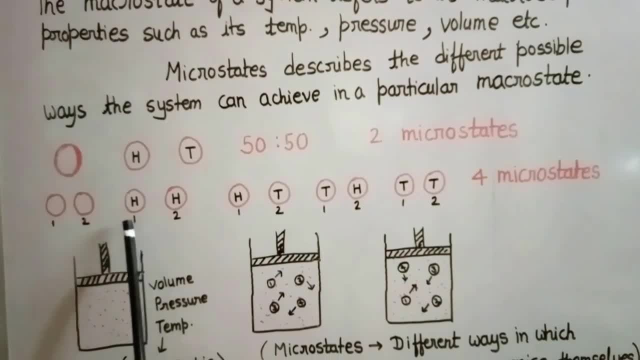 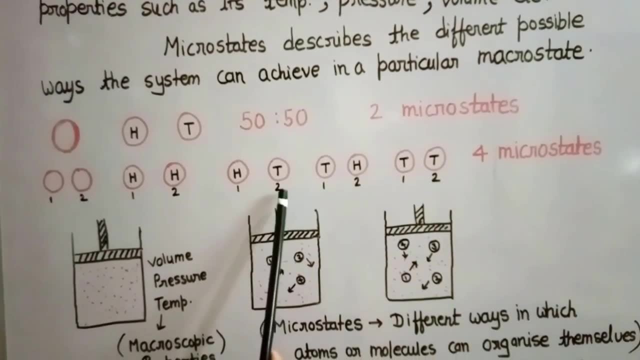 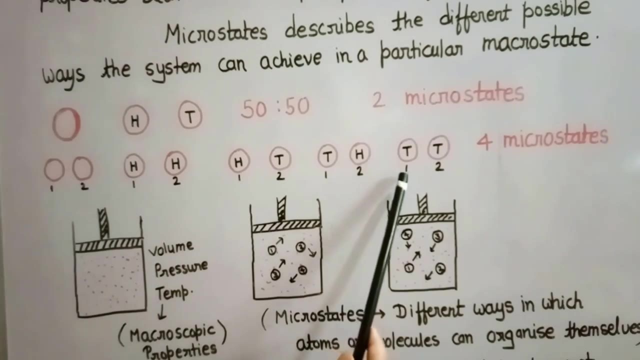 may be that both the coin have had. The another possibility is that the one coin has had and the another coin has still. The second possibility is that the first coin has still and the second coin has had. And the third, fourth possibility is that the both coin can come tail position. So there are 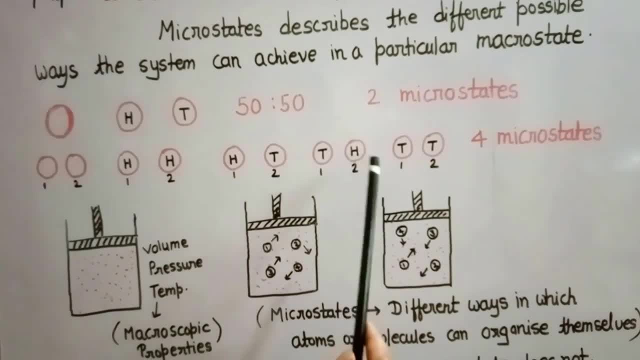 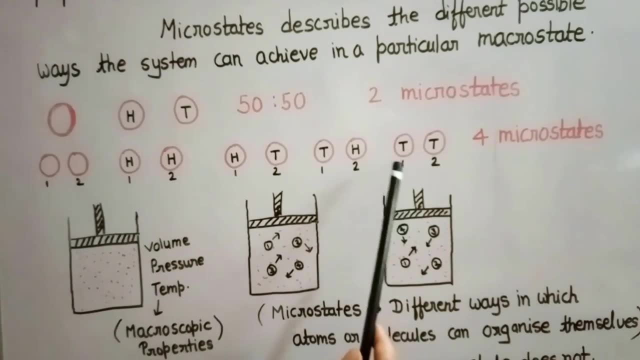 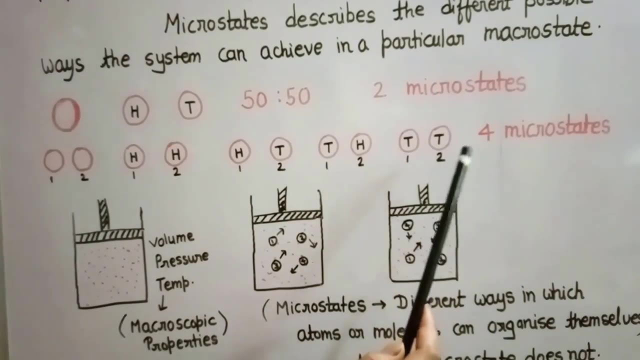 four different ways which the two coins can take. It means there may be four micro states when we see these two coins. It means two coins are the macro state of the system and the four ways that they can take are the four micro state of the system. 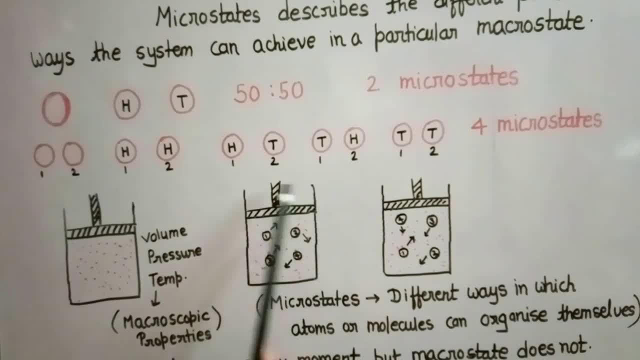 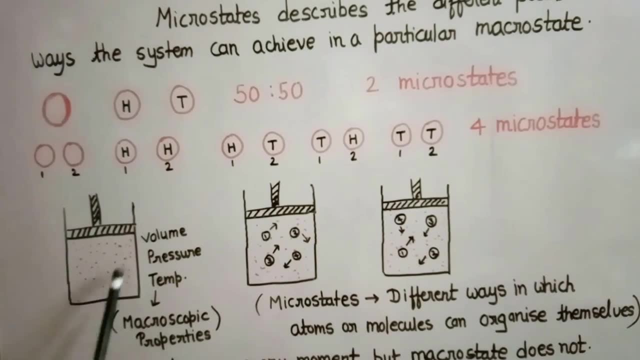 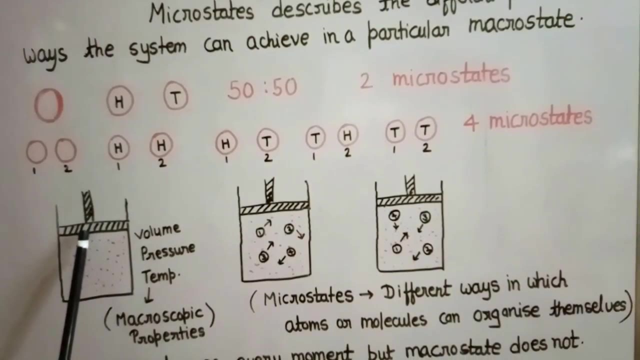 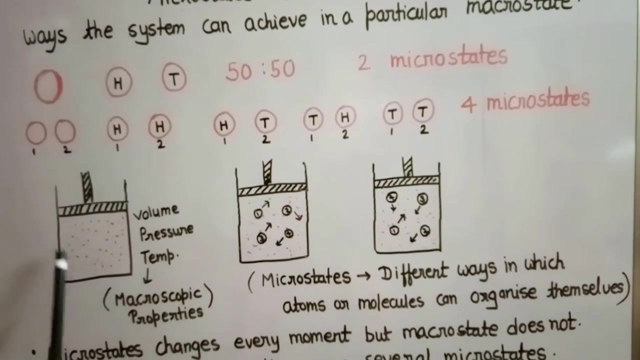 Now it comes to the thermodynamics. In the thermodynamics we take a cylinder And this is a cylinder, and in this cylinder there is a piston. By this piston we can change the volume, the pressure or the temperature of this cylinder. It means, of this gas that is filled inside this cylinder There is a 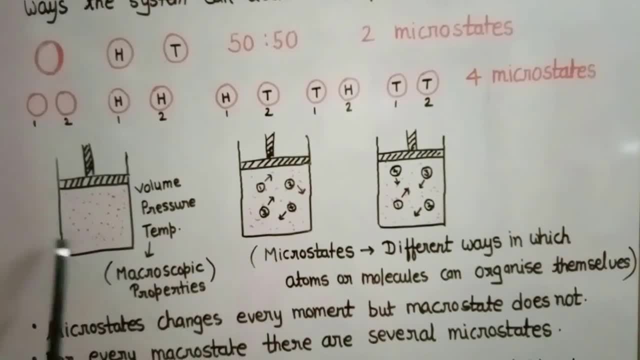 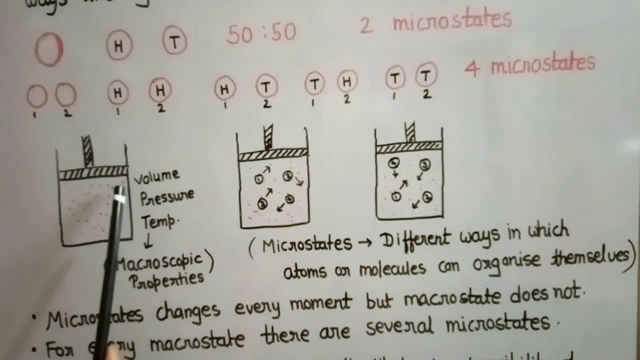 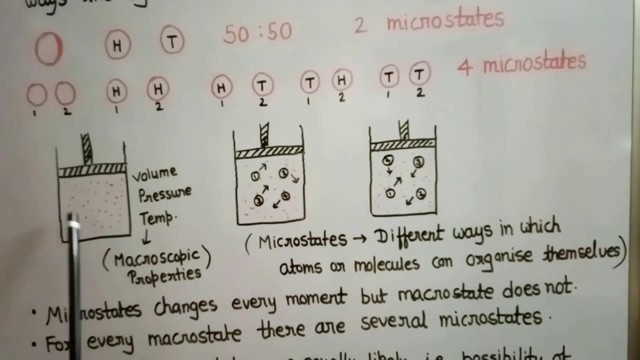 gas that is filled inside This cylinder. so this makes a system. now the macro state of the system can be defined by its volume, or by its pressure or by its temperature. it means its volume may be 1 liter. this defines its macro state. it may have 1 million molecules, this defines its macro state. these are called macroscopic. 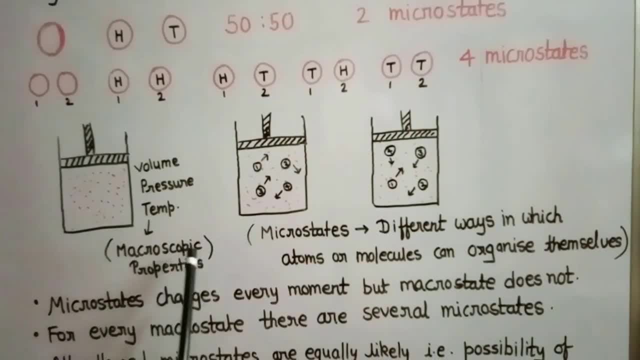 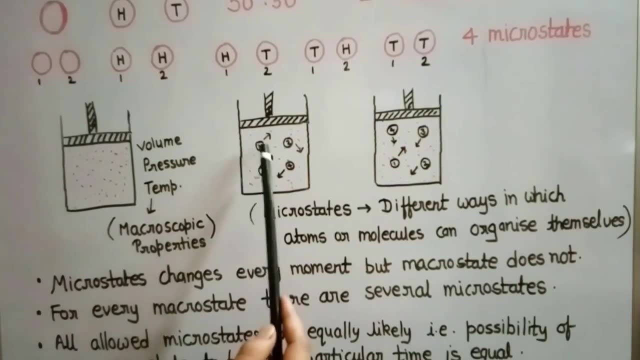 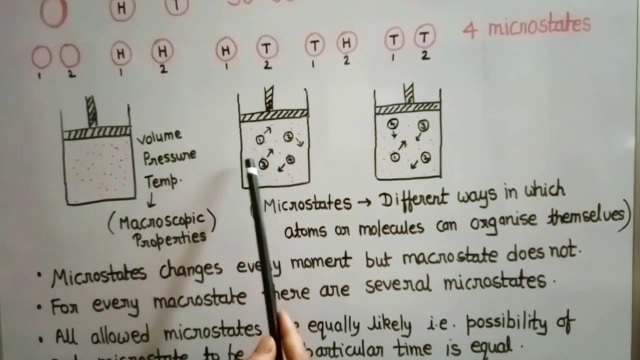 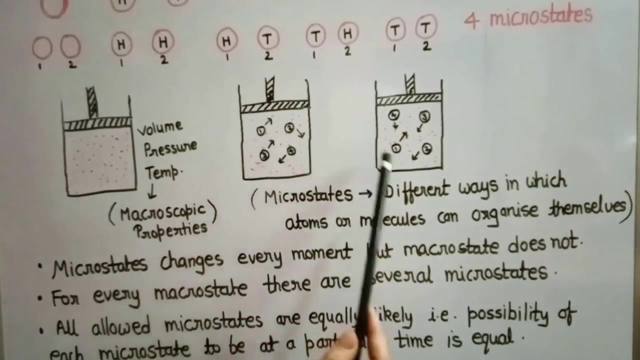 properties. now, when we see deeply this gas, there are so many number of atoms or molecules inside this. these molecules are are rotating simultaneously. each is moving, so it may take different positions at any time. at any time, the first molecule may be here, or it may be here or 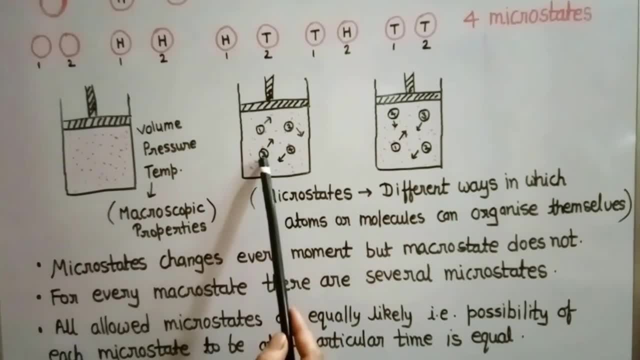 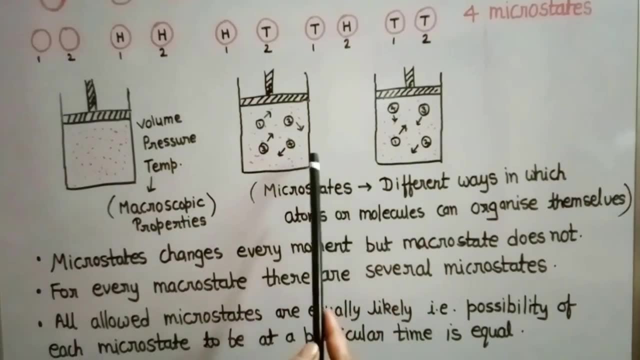 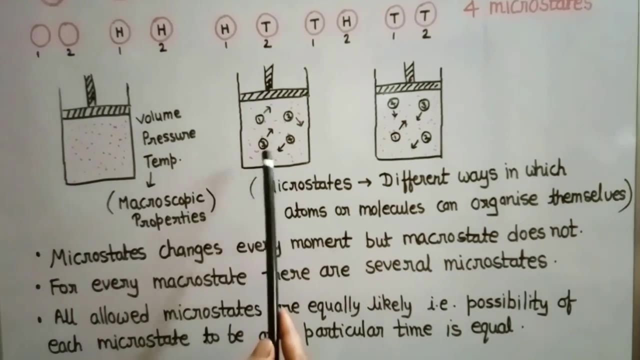 it may be anywhere another position: the third molecule may be here, or it may be anywhere another position: the third molecule may be here, or it may be here, or it may take any other position. so when we see this gas at any time, the position of its molecule may be different and the system can take different. 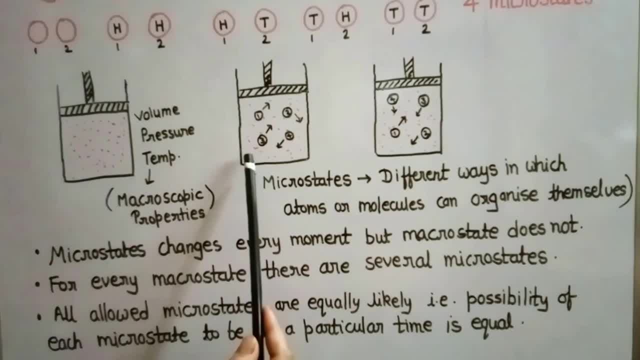 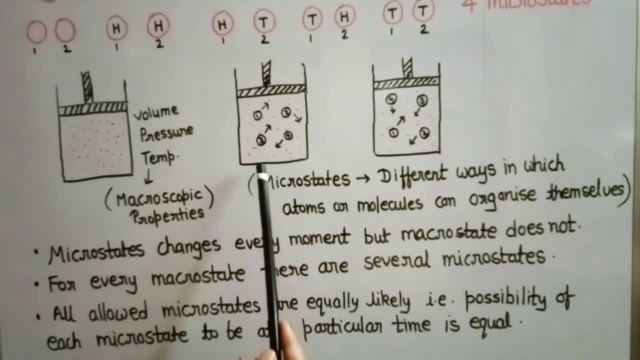 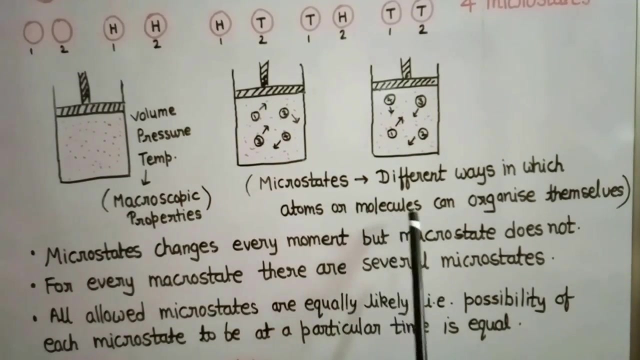 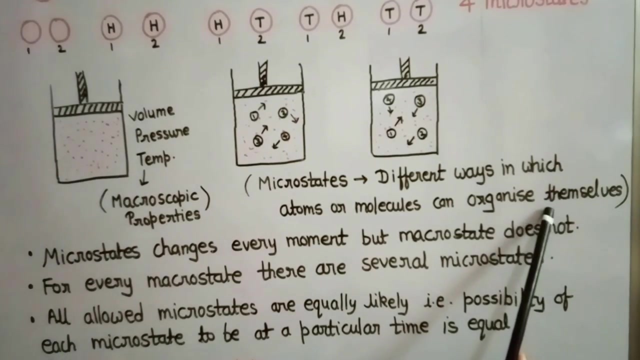 configurations of the molecules. there are so many nice number millions of atoms or molecules are present here, so there may be different ways that the system can take takes. this is call it micro state. so the micro state is the different ways in which the atoms or the molecules can organize themselves. it means how many different ways that they 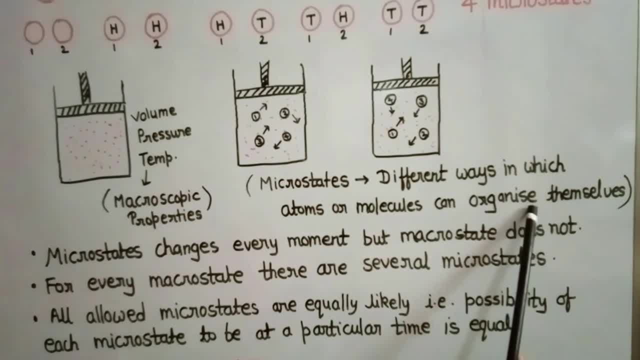 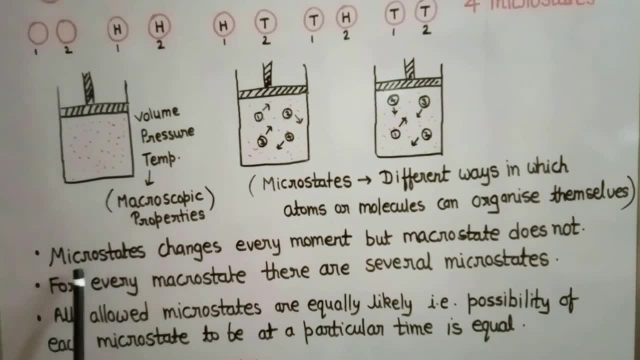 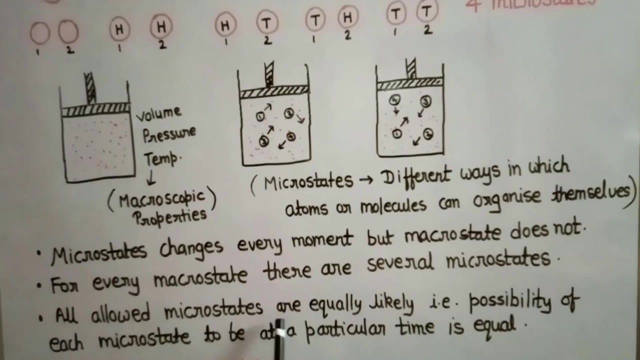 can take. so there may be a large number of micro states for this system. so in general the micro state changes every moment, but macro state does not change and for every macro state there are several micro states and all allowed micro states are equally likely. it means the possibility of each micro state to 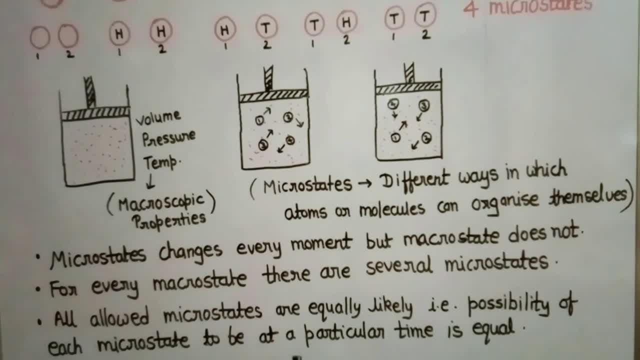 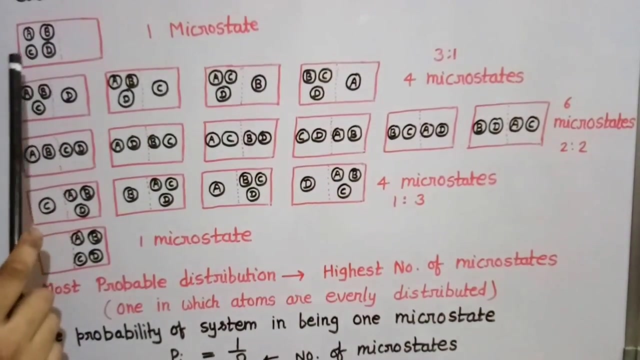 be at a particular time is equal. it means for, for example, if we take a coin, there is equal possibility that the micro state will be equal to the micro state, that the head will come or the tail will come. now we will understand this by another example. now, in this example, we can have a compartment. 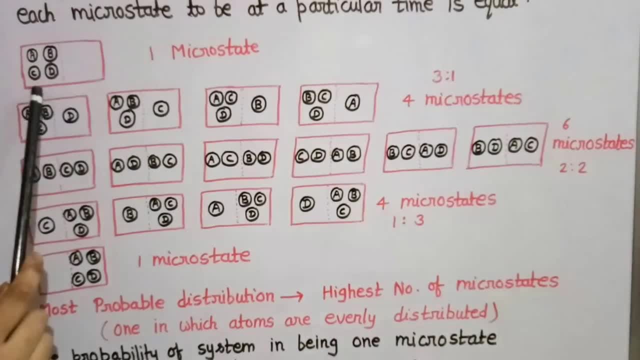 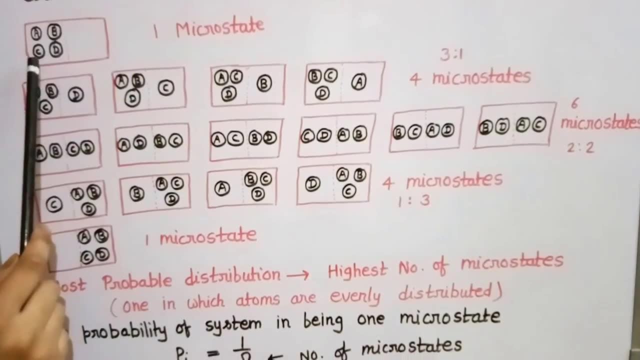 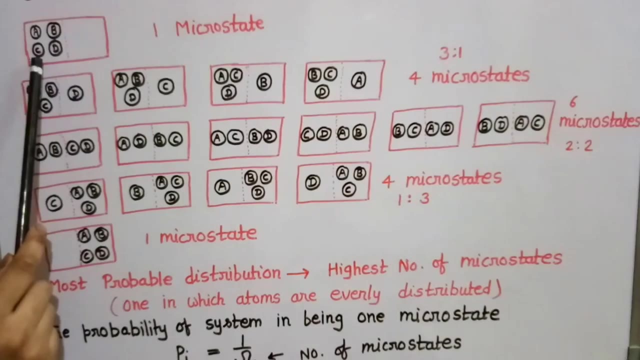 like this, and this is divided into two chambers: first chamber and the second chamber. now, the first possible way may be that the all four atoms ABCD are divided into two chambers, and the first possible way may be that the all four atoms ABCD are present in the first compartment. there will be only one way that the molecules 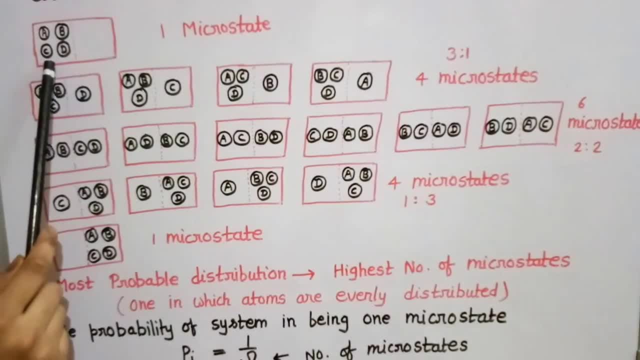 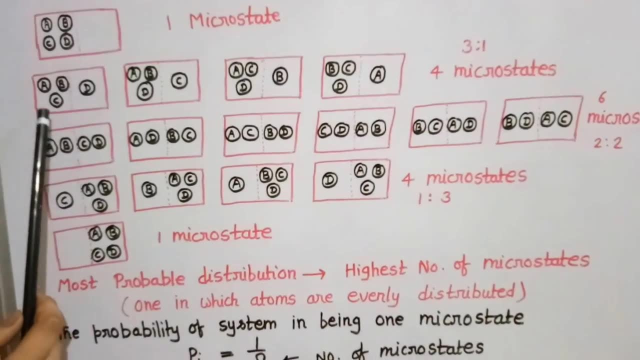 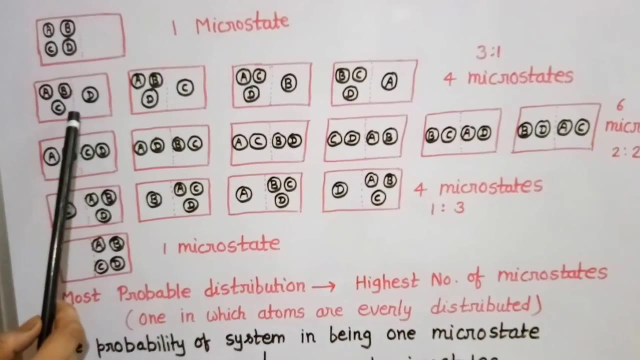 can take when they are in one compartment, so it will have one micro state. the another possibility may be that the three atoms on molecules are in first compartment and one atom or molecule is in the second compartment. this may have four probabilities. it means first probability: maybe ABCD are in worst. 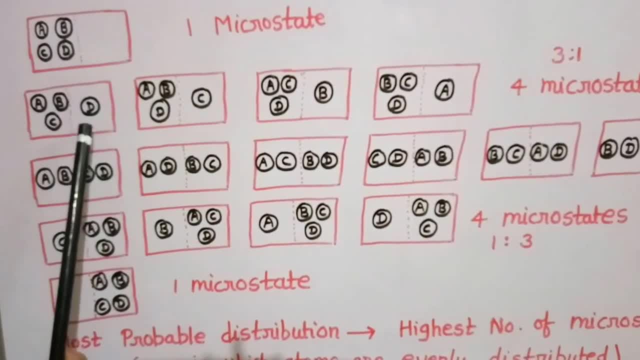 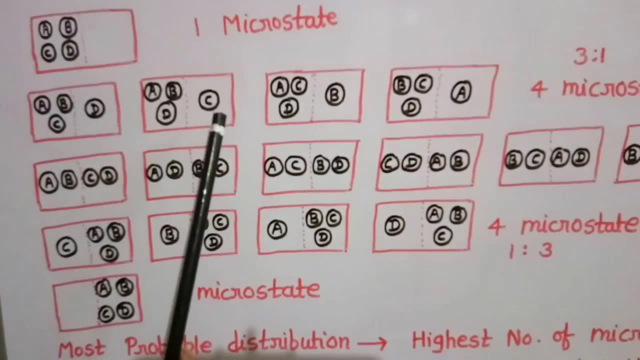 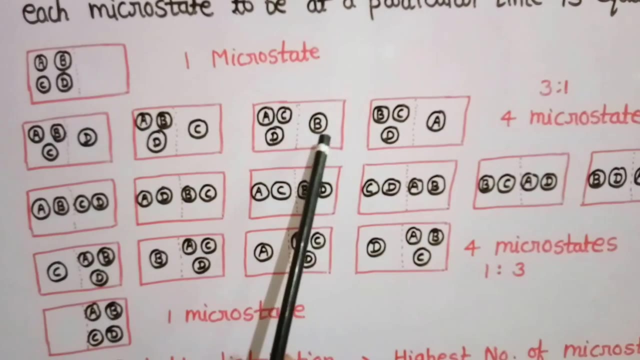 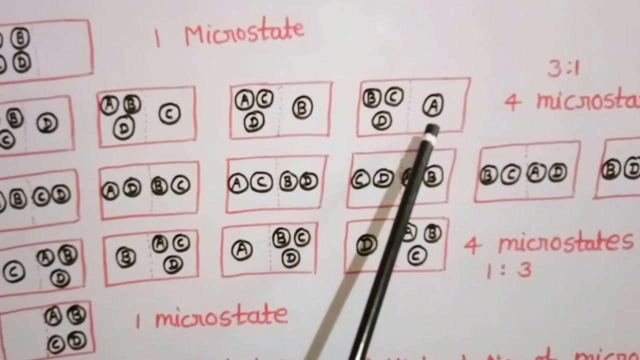 compartment and D in the another compartment. it may be a, B and D in the first compartment and C in the second compartment. it may be a CD in the first compartment and B in the second compartment, or it may be B, C and D in the first compartment and a in the second compartment, so there may be four. 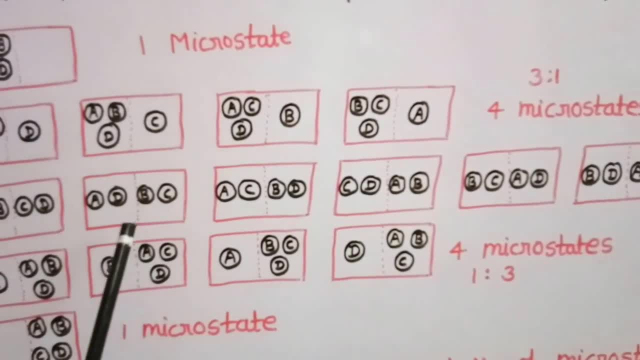 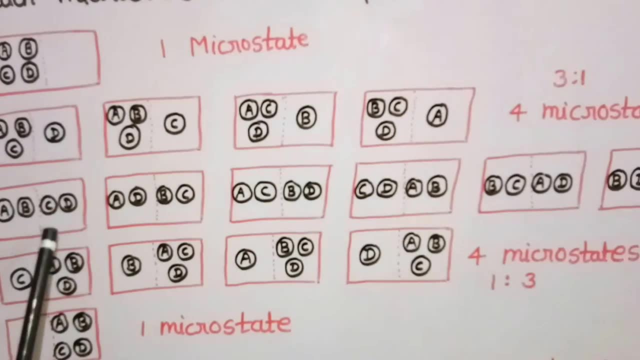 microstates in this condition. the third possible way is that there are two atoms or molecule in first compartment and the two letters are molecules in the second compartment. this may have six types of configuration. the first maybe A and B in first and C and D in the second compartment. the second is a and D in the. 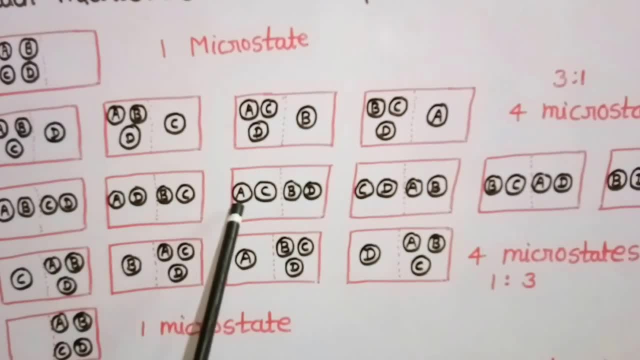 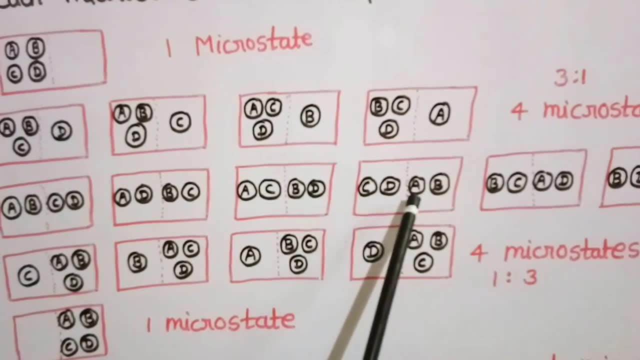 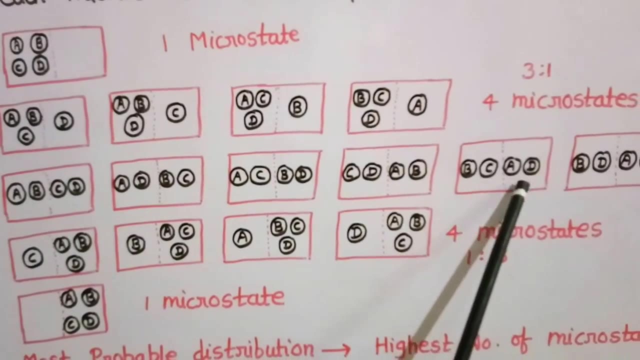 first and B and C in the second compartment and C in the first compartment and B and D in the second compartment. C and D may be first compartment and A and B in the second compartment. B and C in the first compartment and A and D in the second compartment and B and D in the first compartment and A and C. 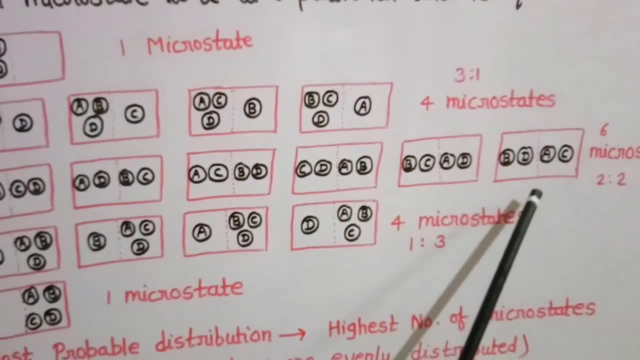 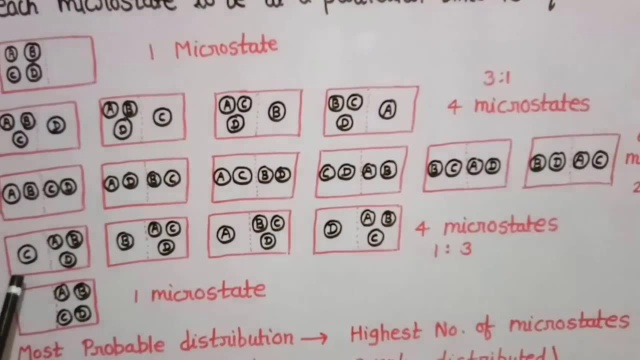 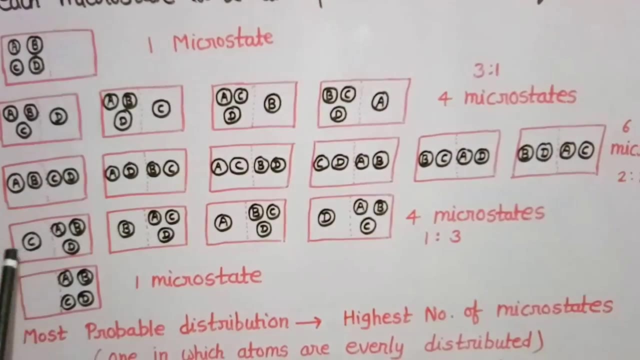 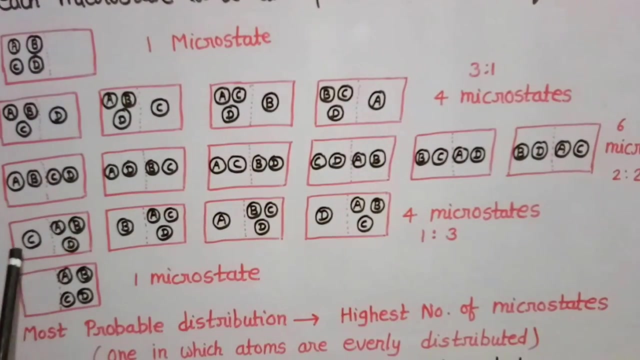 in the second compartment. so there are six microstates possible for this configuration. the fourth may be the one molecule or atom in the first and the three molecules or atom in the second compartment. so this will like this and it will also four different microstates. it means C may be in first compartment, B may be in first compartment, a may be in first compartment. 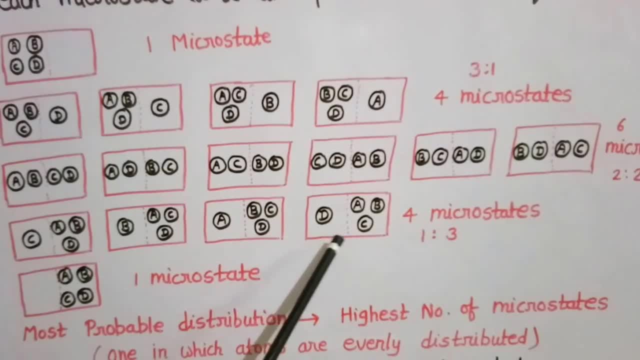 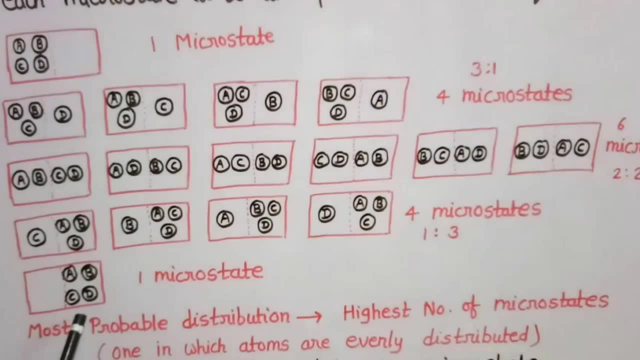 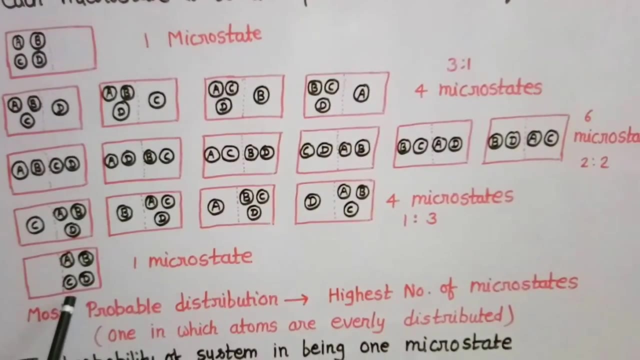 and D may be in the first compartment. so this will have four microstates. and the last way may be that all the four atoms or molecules are in the second compartment. it means all A, B, C, D in the second compartment. this will have only one possible way and it will have 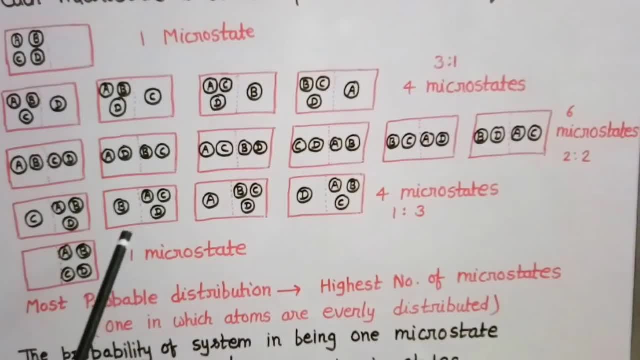 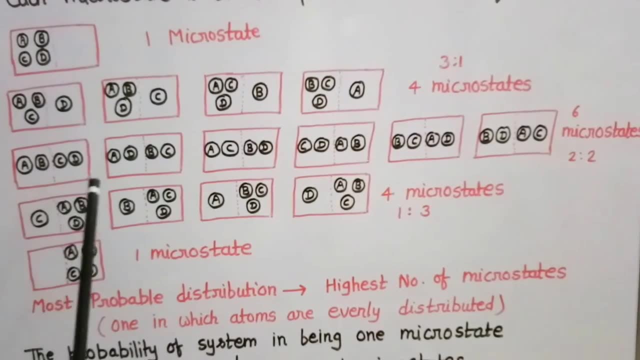 one microstate. so from this picture we can see that the highest probability will be found. highest distribution is found when there are six microstates. it means this is the most probable distribution. when the atoms are evenly distributed, it means half and half distributed between both compartment. so we can say that the most probable distribution is one that will have. 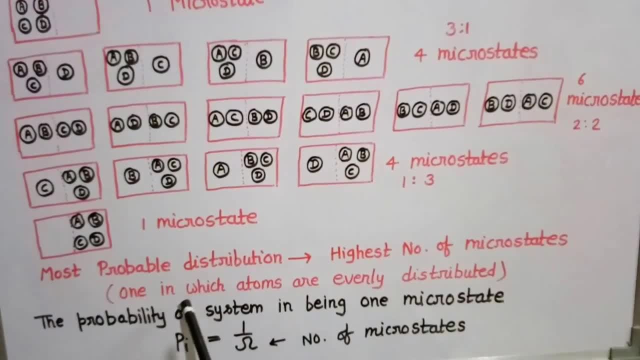 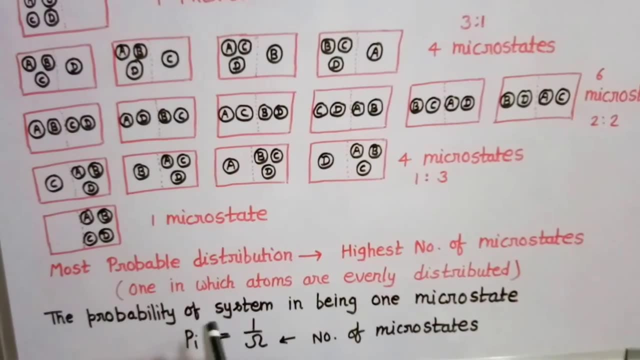 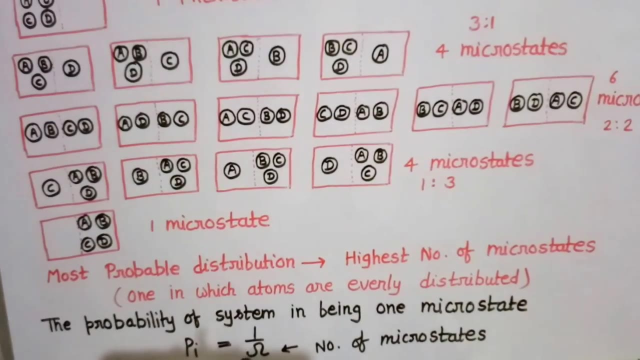 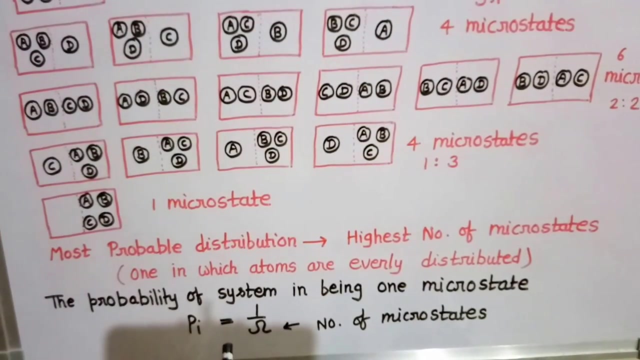 highest number of microstates. it means one in which atoms are evenly distributed and now the probability of the system is being one of the microstate. it means probability will be equal to 1 upon omega, where omega is the number of microstates. now the microstates are related to the entropy. 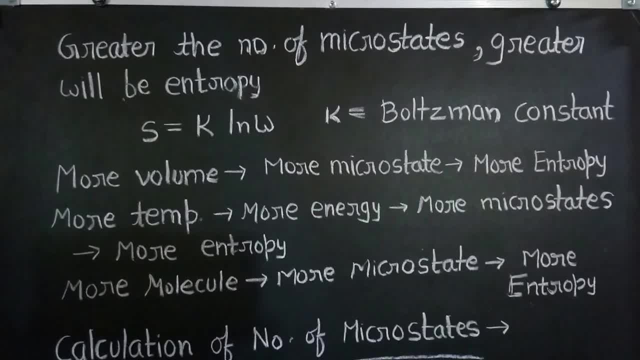 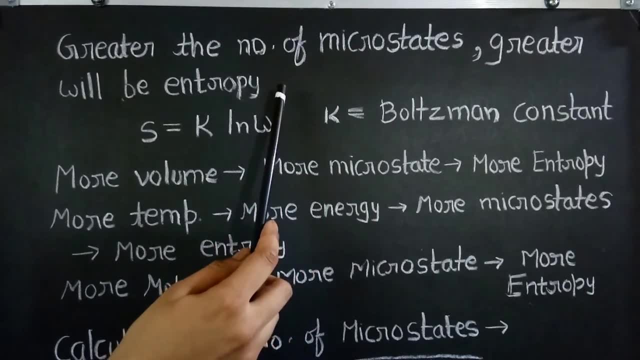 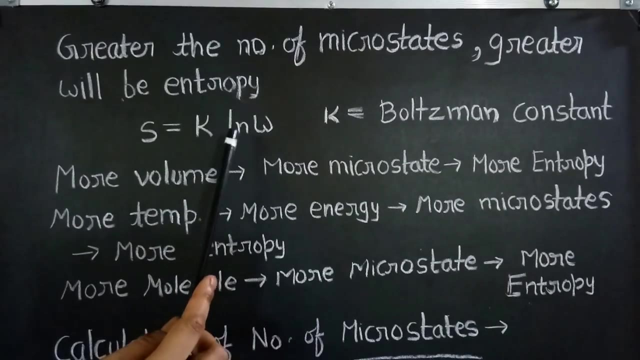 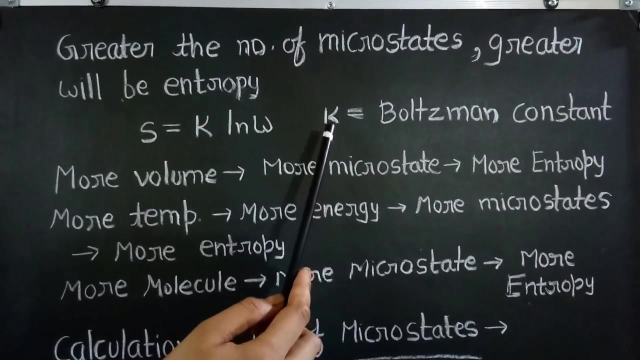 actually, probability is related to microstates and microstate is related to entropy and as greater the number of microstates, greater will be the entropy. volksmann, a scientist, given a relationship between entropy and the number of microstates, or probability that is, s is equal to k, ln, w, where k is the volt span constant, its value is 1.38 into 10, raised to. 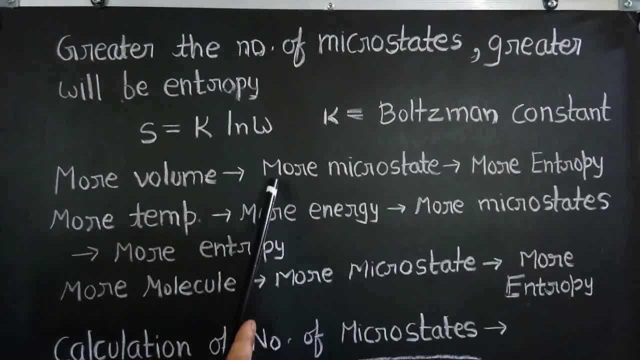 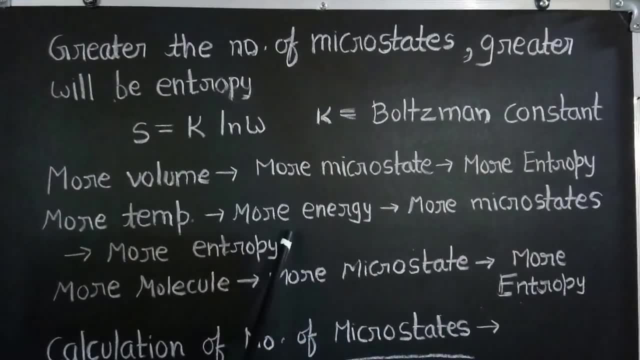 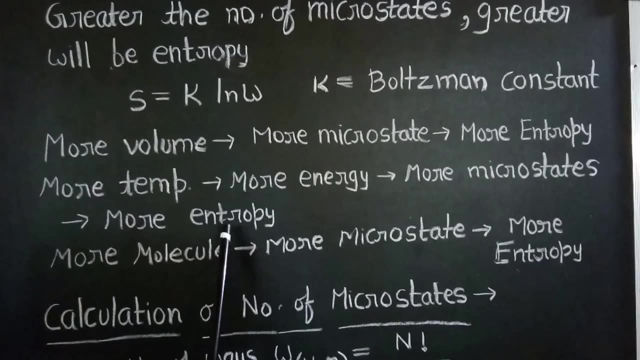 the power 23, so more will be the volume, more will be the microstates and hence more will be the entropy. and when more is the temperature, more will be energy, more the molecules will move and more will be the microstates and hence more will be the entropy. similarly, more the molecules, more will be arrangements. 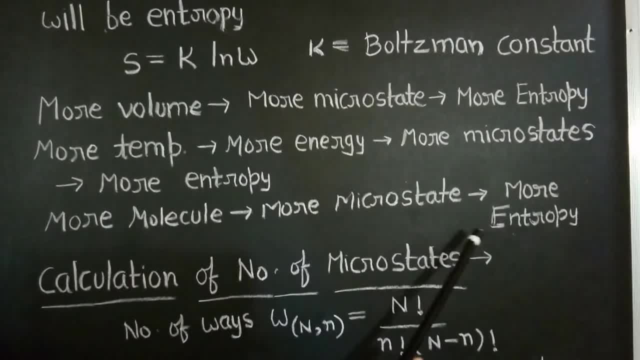 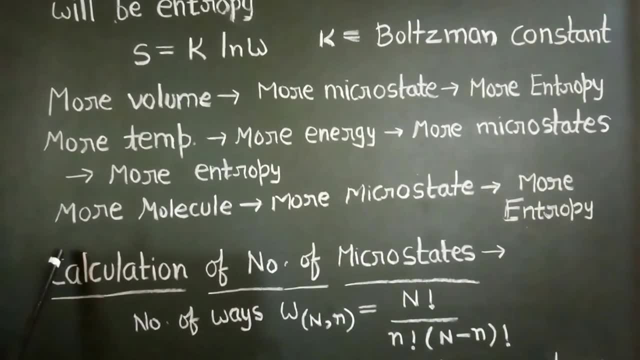 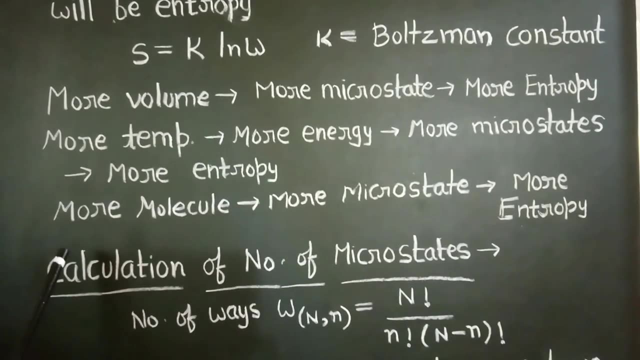 and more will be the microstates and hence more will be the entropy. now we comes to the calculation of number of microstates, as this is the smaller case we have studied in which we can count the microstates, but there are a lot of number of atoms or molecules in a solid that we cannot count, so we 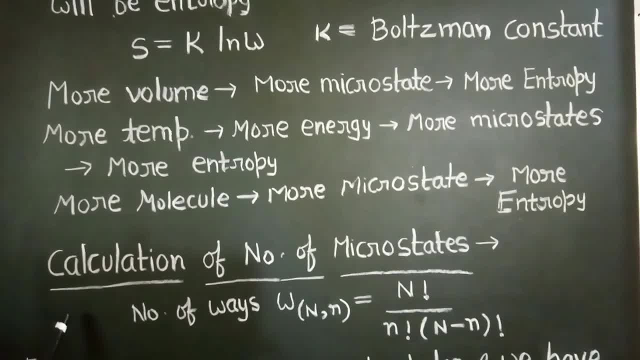 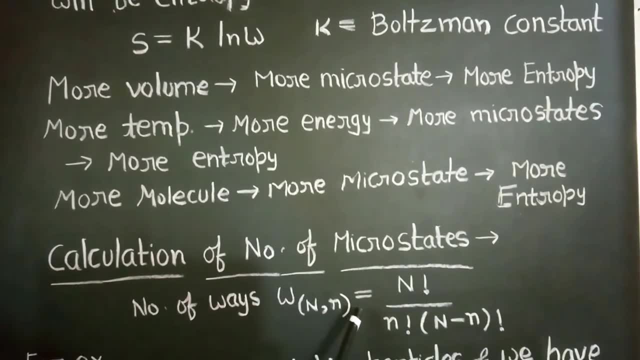 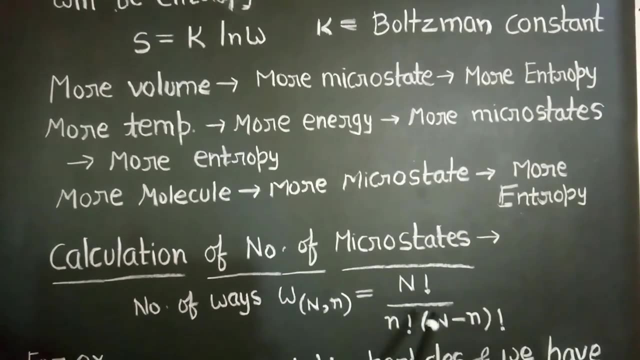 will make a formula to calculate the number of microstates that is given by number of ways: w and n is equal to n factorial, upon small n factorial and minus small n factorial, where n is equal to the total number of particles and small n will be the specific or the special number of particles that 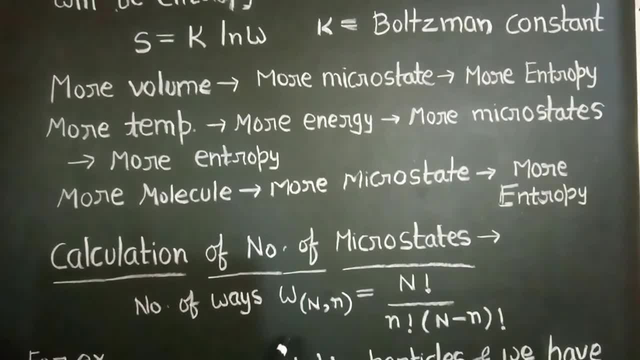 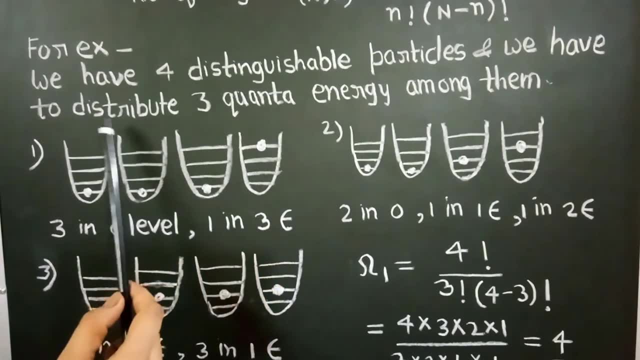 a special position. we will understand it by an example. we have four distinct usable particles and we have to distribute three quanta of energy among them. then there we. there will be three possibilities, three different ways that the atoms can take space. this is the energy level diagram. 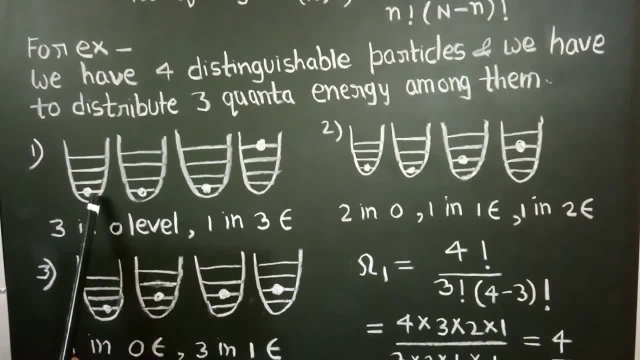 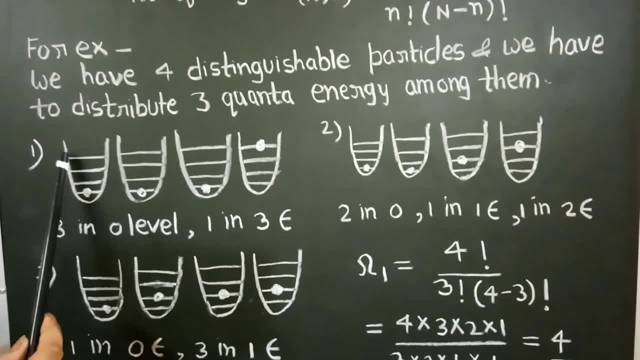 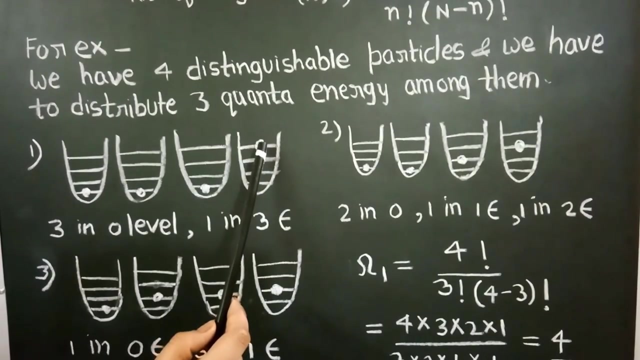 for an atom in which the first level represents the ground level. this represents the first excited state, this represent the second excited state and this represents the third excited state. so the first possibility may be that the three particles are in the ground level and the one particle is in the third excited state. the second probability may be the two articles. 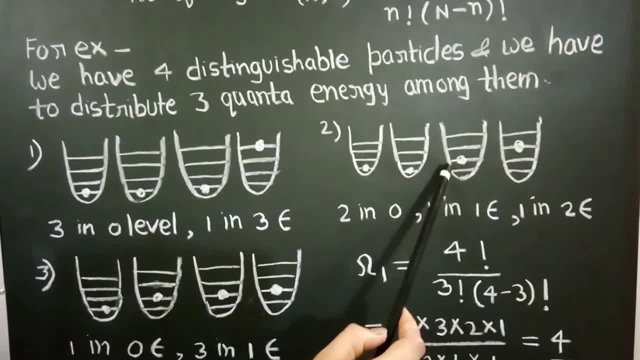 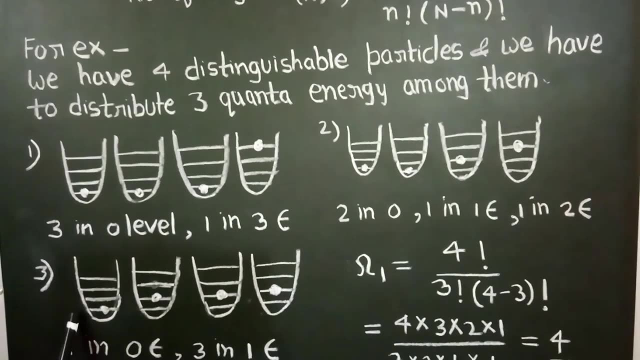 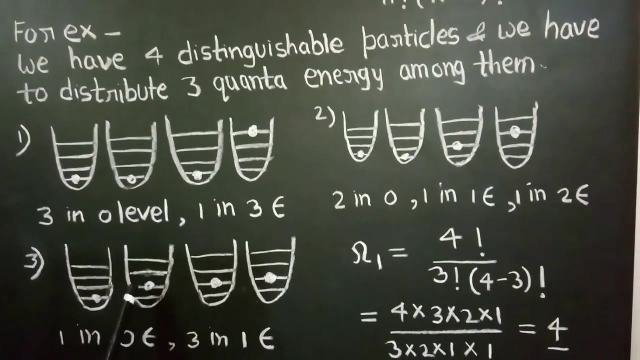 are in the ground level. the third particle is in the first excited state and this particle, the fourth particle, is in the second excited state. the third possibility may be the one particle in the ground state, the second particle in the one at first excited state, this particle also in the 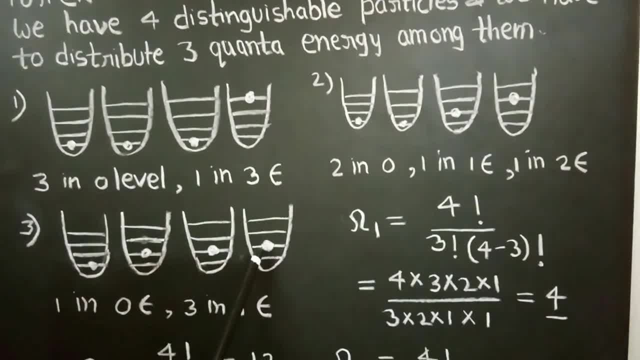 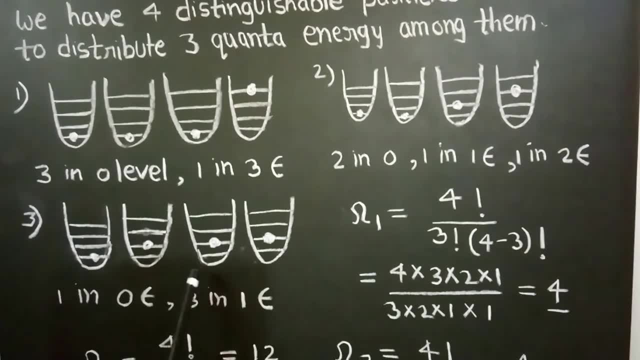 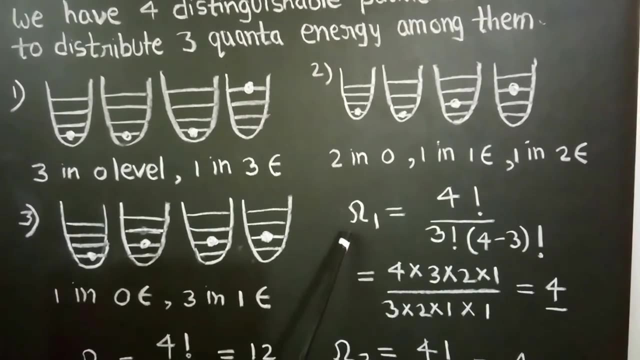 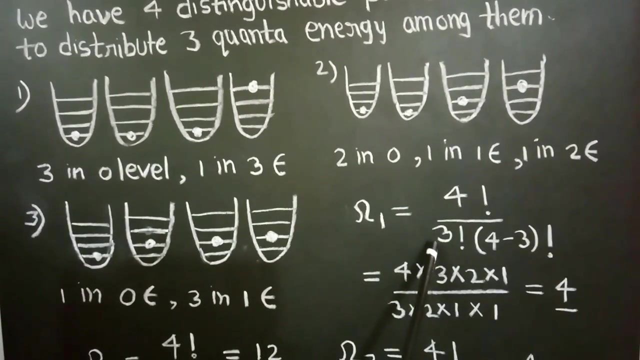 first excited state, and this also in the first excited state. it means one in the ground level and three first excited state. so in the case of this, in the case of first possibility, the number of microstates Omega 1 will be equal to 4 factorial upon 3 factorial, 4 minus 3 factorial. so how to solve the factorial? 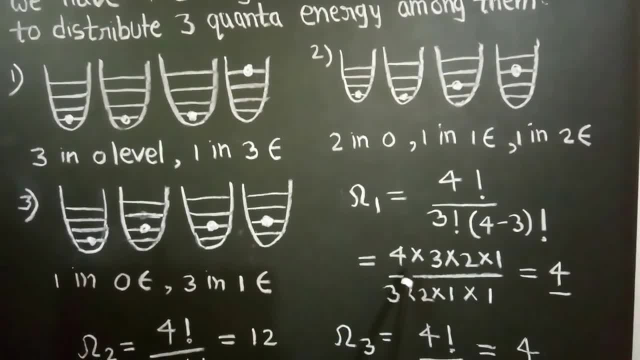 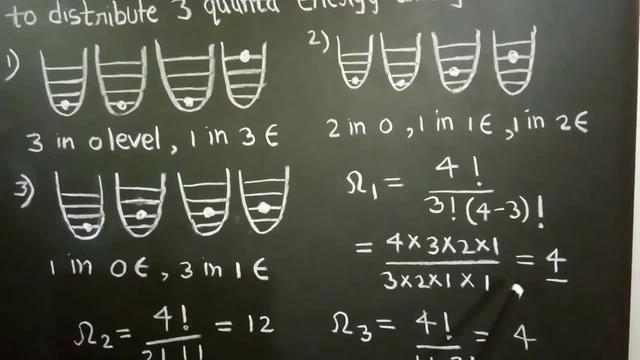 we live. we did it like this: 4 into 3, into 2, isn't it into 1 upon 3 into 2 into 1, into 1 is equal to 4.. So there will be 4 number of microstates. It means 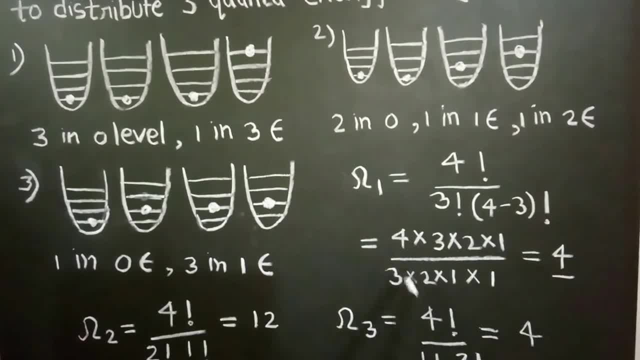 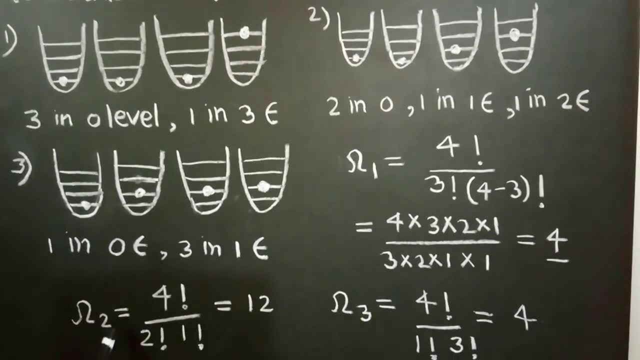 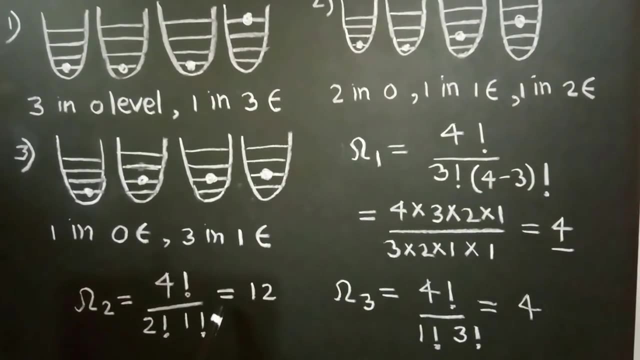 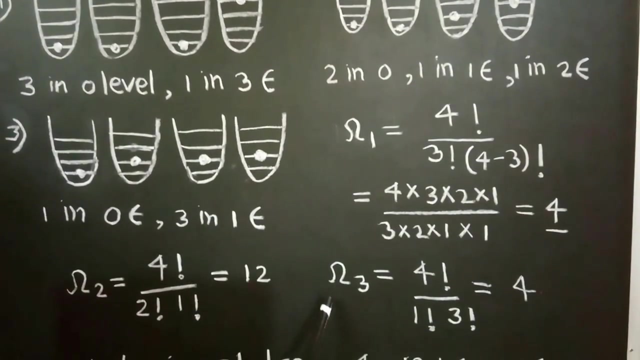 4 possibilities, 4 different ways. In the case of this second possibility, the number of microstates will be: omega 2 will be equal to 4 factorial upon 2 factorial, 1 factorial, and it will give 12 microstates. The third possibility: it means the third number of microstates will be: 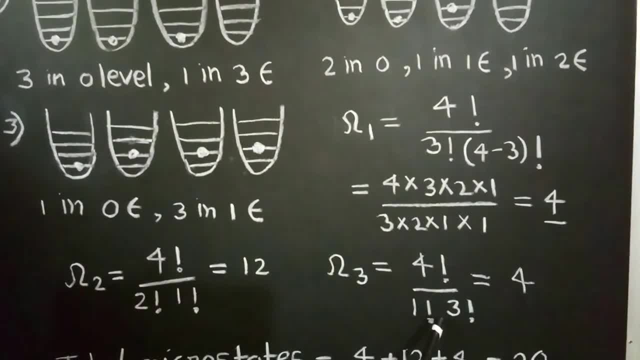 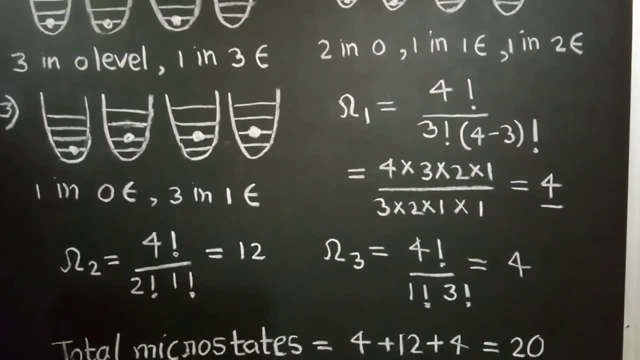 4 factorial upon 1 factorial into 3 factorial and it will give the value equal to 4 microstates. So the total number of microstates will be 4 plus 12 plus 4 is equal to 20.. In the similar way, 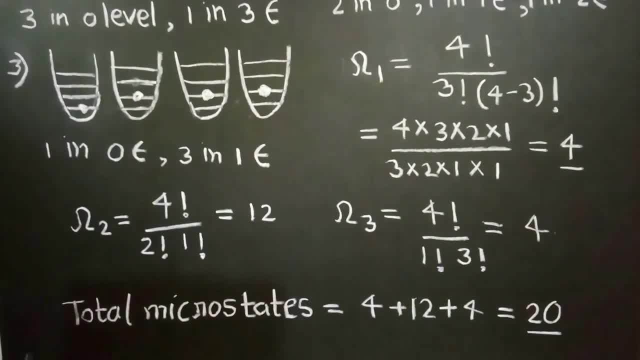 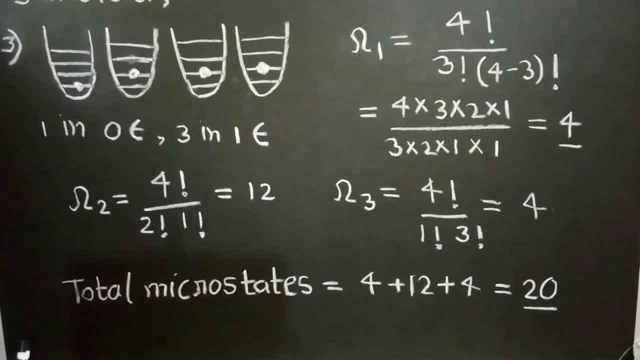 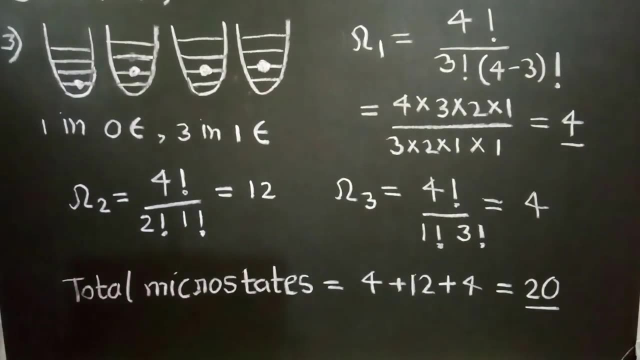 we can solve any question and we can calculate the number of microstates. in any case, If you have any problem, you can comment us. If you like this video, please comment. please like this video and please subscribe our channel. Thank you.